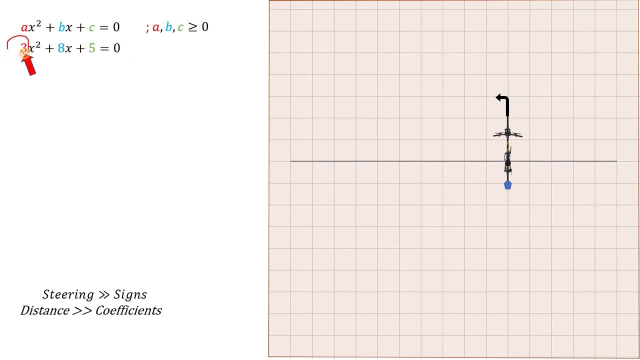 bicycle. so let's first start with this number three. so this number three represents three-unit distance that is covered by the cycle. so we move three units in the bicycle: one, two and three units. then we have already addressed the path of three X square. then comes the turn of this plus sign, as we already said, that the 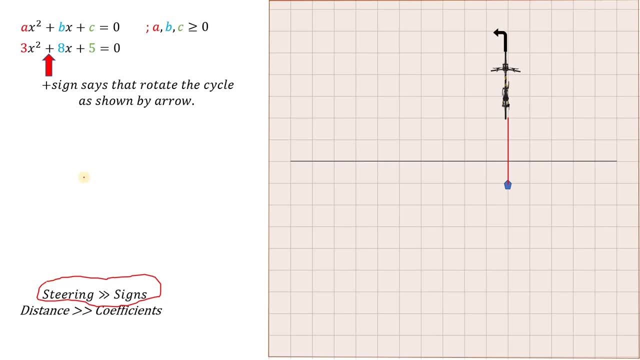 signs represent the steering or the handle. so the plus sign says that: rotate the cycle as shown by the arrow. you can look here. this arrow is pointing in this direction, so rotate this bicycle in that direction. then comes the turn of eight. so eight means the coefficient. so we cover the distance of eight units by. 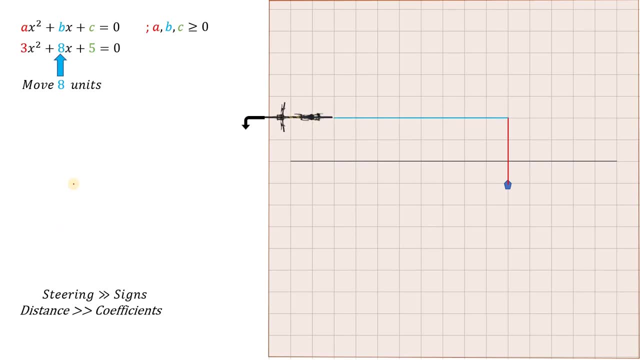 using the cycle. then, similarly, turn comes for this positive sign. so the positive sign says that rotate the cycle as shown by the arrow. so this arrow is going in this direction, so rotate it. then the turn of five comes. then move distance of five units by riding the bicycle. at last, what you do. 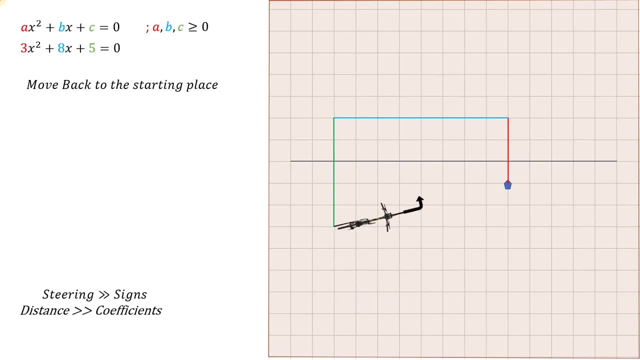 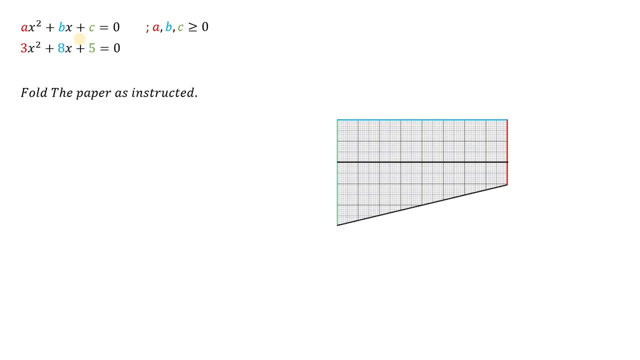 is just move back to the starting place like this: by doing this process, you have made a quadrilateral. so in the next step you cut this quadrilateral out of the graph paper. then it will look like this: then what do you do is you fold the paper as instructed. so this is the paper we have got. now I'm using a. 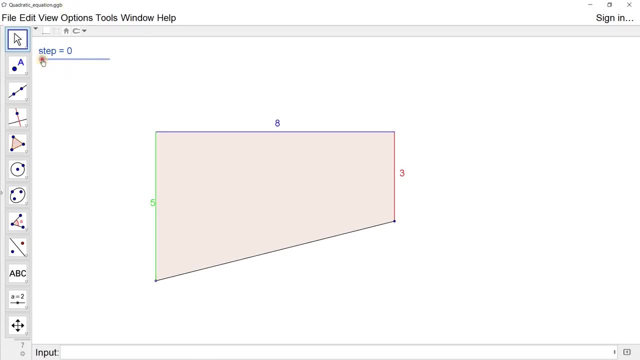 software called GeoGebra to fold this paper. so in the first step we fold the paper in half such that it adds crease at the middle. for doing so, I'm going to fold this paper just in half like this, so that it will add a crease at the. 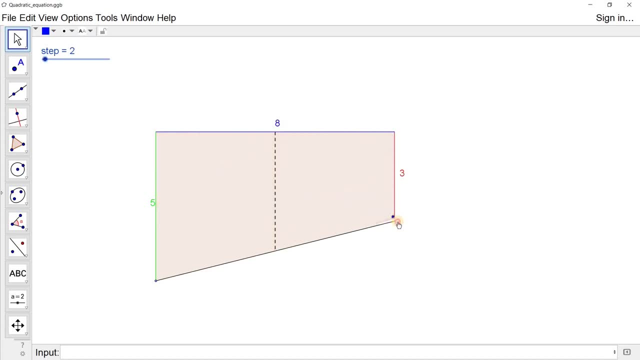 middle. so just unfolding it will get a crease like this in the center. then in step three, what we do is bring the bottom corners to the top blue line by folding, but by putting from the midpoint. what it says is: let's bring this top most corner to touch this blue line in such a way that the bottom most corner 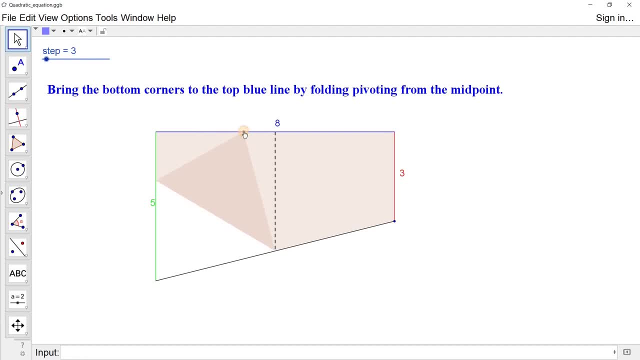 just touches the mid crease over, like this, and the same process is done for this point also: just fold the paper in such a way that it just touches the blue line and at the bottom it just meets the middle crease. so then what we do is mark these two points. so these two points are what we get as a result. now, 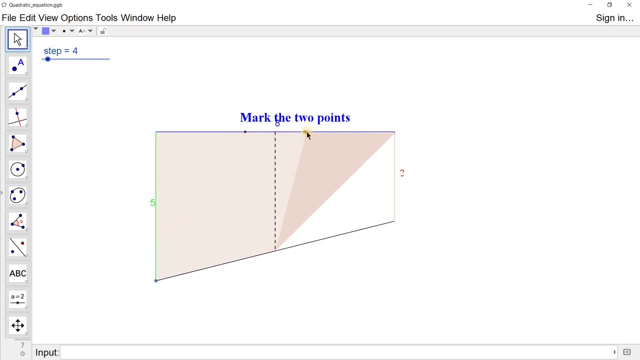 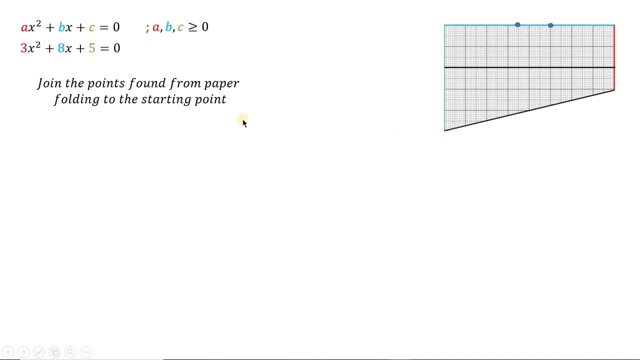 let's unfold the paper again. let's unfold the paper. so these are the two points that we got after folding the paper. now what we do is join these two points to the starting point. this is the starting point. join the first line and join the second line like this: now measure the two distances and they will. 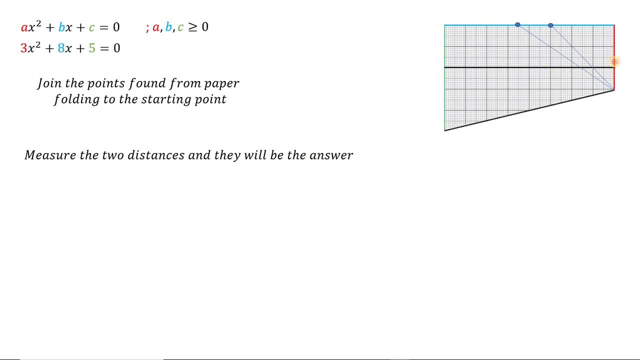 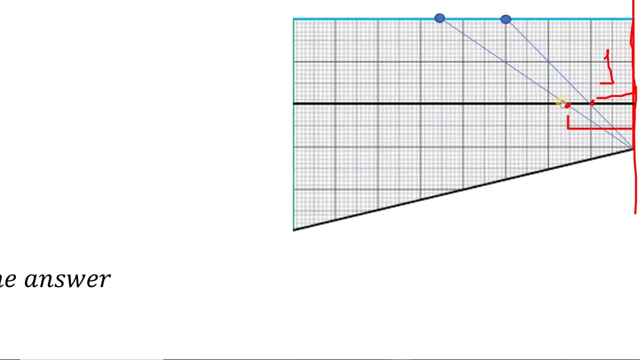 give the result to measure the distance. you measure the distance from this red line straight to this point, so this will be 1 units, and you also measure the distance from this point to this point, which you can clearly see. it's almost greater than 1.5, so it's almost 1.7. 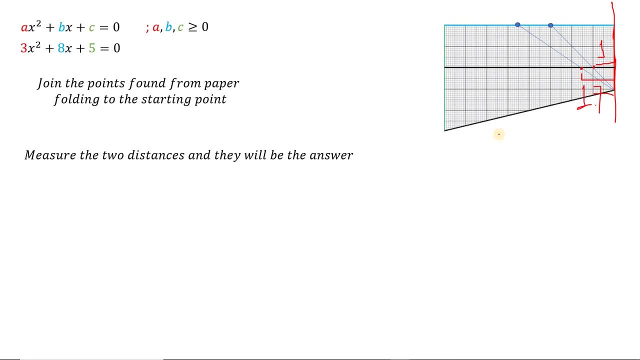 units. so 1 and 1.7 must be the result. but you can see that these distances are on the line left side of this red line. so, as you can see in coordinate geometry, if you look in the left direction it will give the negative results. so negative 1 and minus. 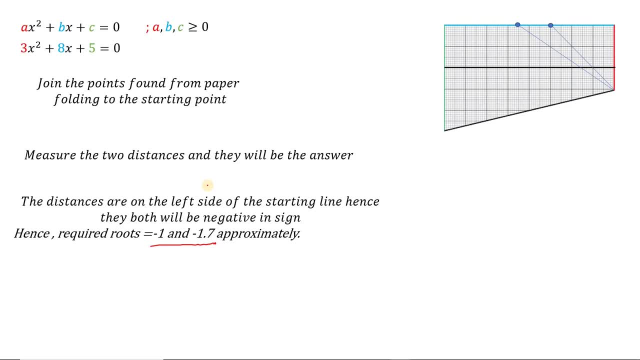 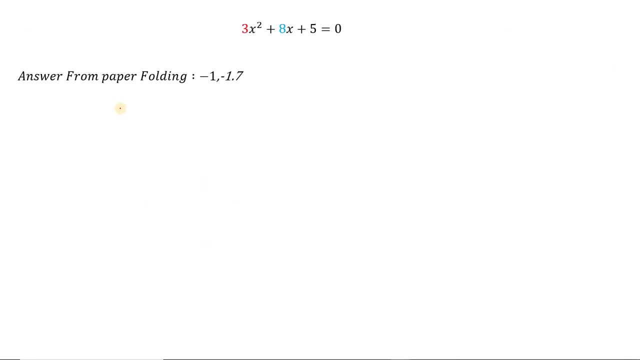 1.7 are the approximate results that are given by the paper folding technique. but you might have some question, because the answer that we get from paper folding is minus 1 and minus 1.7. but by using the real algebra we get the result to be minus 1 and minus 1.6667. so are we doing something wrong in origami? 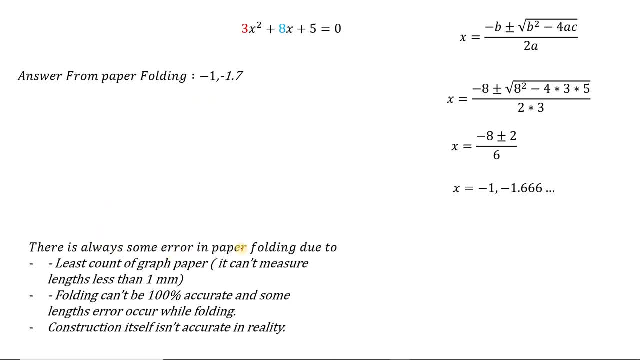 so the answer is there is always some error in paper folding. one reason is the least count of graph paper because it cannot measure the lengths less than 1mm and folding cannot be 100% accurate and some lengths error always occur while folding. and the main reason is construction itself isn't accurate in. 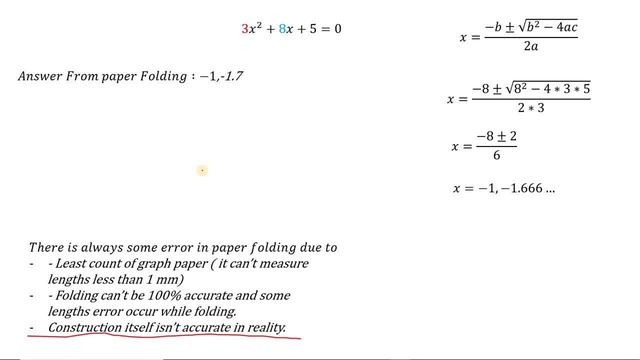 reality. let's say an example. suppose you want to draw 5 centimeter by the ruler in a paper, but you can't be sure whether the measured length is accurately 5 cm or not, because it could be something like 5.02 cm or 4.99 cm. 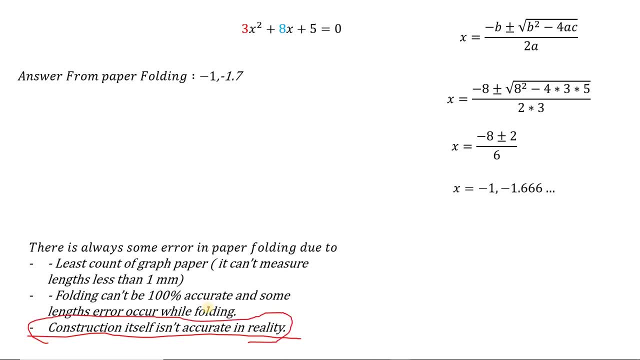 so construction itself isn't accurate in reality. so that's the reason why we don't get the exact result from paper folding. but if you have some ideal situations, like ideal folding, or some software that does some folding, as we did in Geo Zevra, so then this will give the exact result. 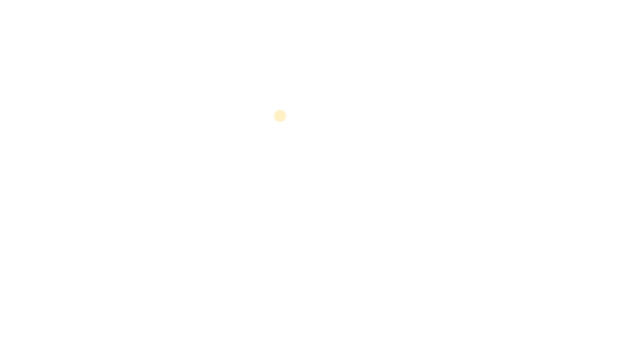 so let's make a slight change in the previous question and make it like this. so let's make a slight change in the previous question and make it like this, so that the second coefficient is negative instead of being positive. so I'll take the same example with the same coefficients, but I will change the sign. 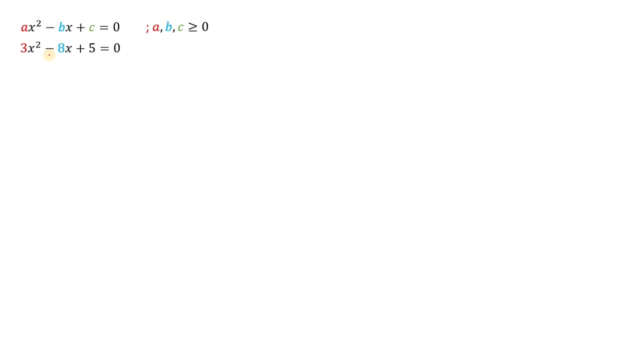 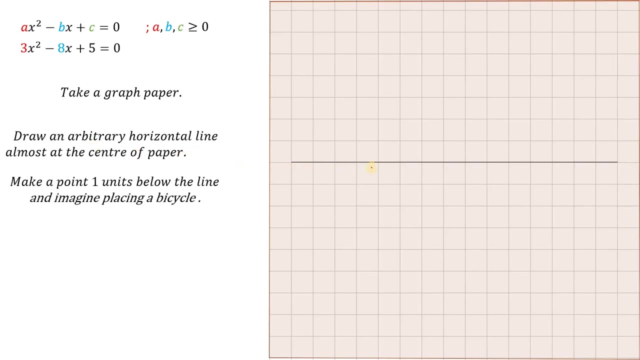 of this 8 and let's see what happens. we'll start from the, so we'll start sequentially from the beginning and we will proceed and we will see the changes in it. so first we take a graph paper, draw a horizontal line, then mark a point below the line and imagine playing a bicycle. then, as we have, 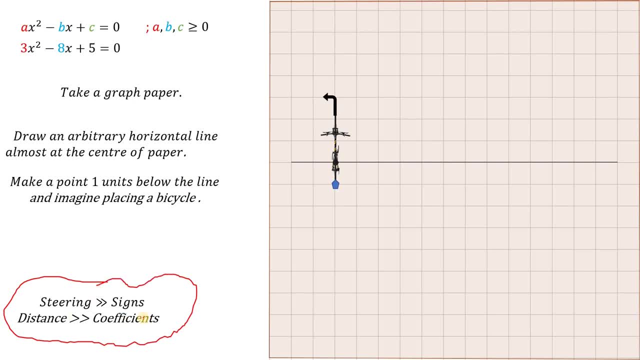 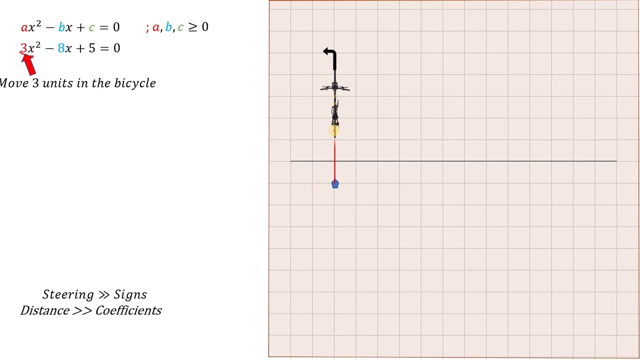 already discussed stillings, Fashion, Ordinaires by science and the distinct, even other coefficients. so at first we will move three units in the bicycle like this. then the turn comes off. negative sign. so here comes the change. negative sign says that click the arrow and rotate as far as 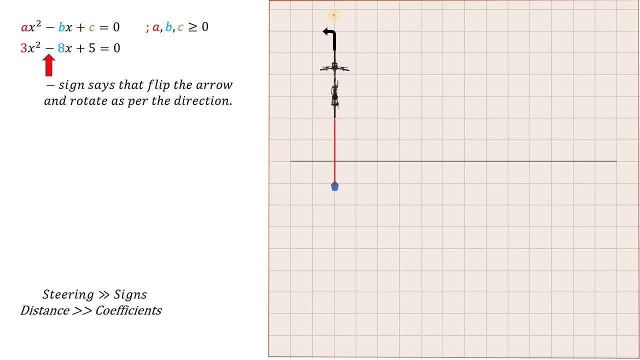 the direction. so first we flip this arrow like this and rotate, so the rotation will be in this direction, now onwards, so it's the turn of it, so a distance, then the turn of positive sign. it says that, it says that rotate the cycle, so like the arrow, so in this direction, and again the turn of five. 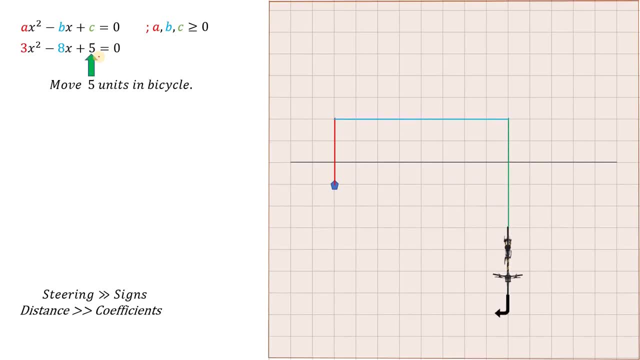 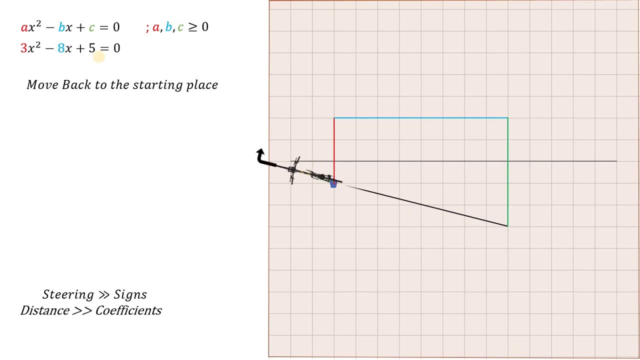 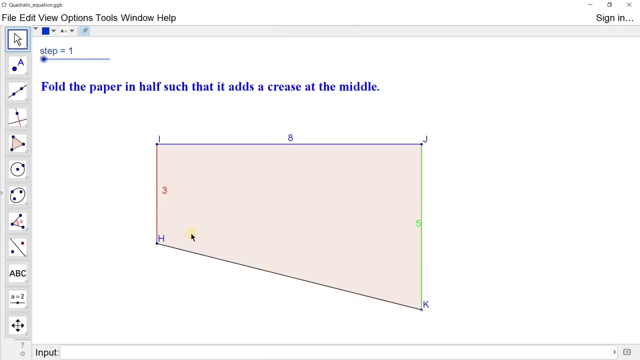 comes. so move a distance of five units, and then you're done. then move back to the starting place where you began, then cut the quadrilateral. at first we fold the paper in half as usual, so then this will give a crease like this. then we unfold the paper, then we bring the bottom corners to touch the. 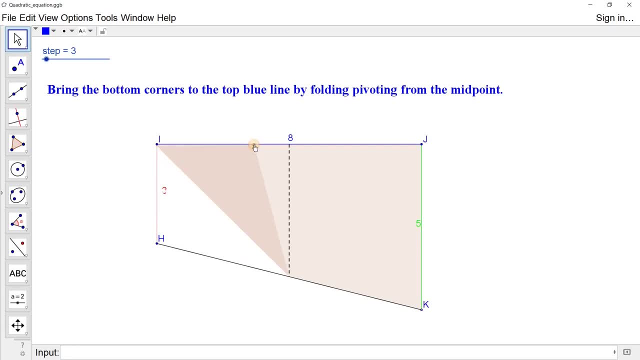 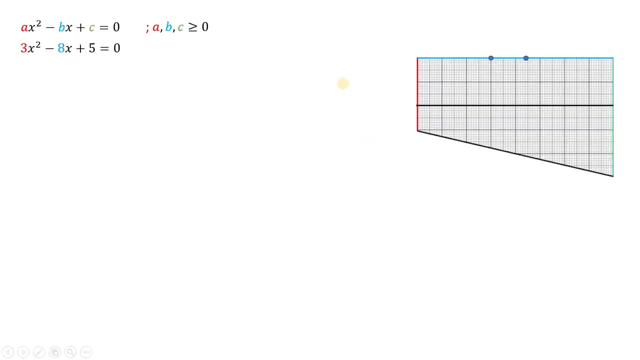 blue line and also touching the middle crease simultaneously. same with this vertex we bring to the blue line and then just touching the middle crease, like this. so in step 4 we mark these two points and again unfold the paper like this. so these will be the two marks thus obtained. so after folding, 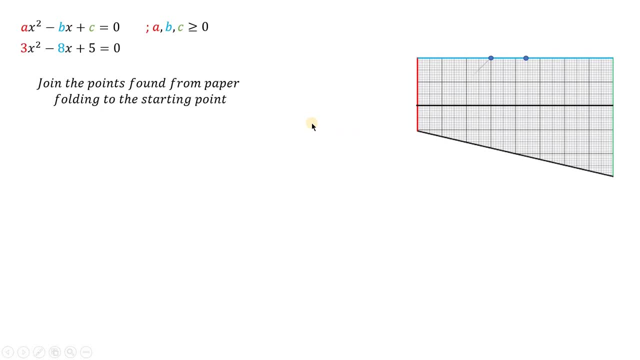 we get these two points, then, as previously done, we are going to join these points to the starting point, as this is the starting point in this case. as you can see now, we measure the distance from here to here, which is one, and we measure the distance from here to this point, which is one. point seven, as